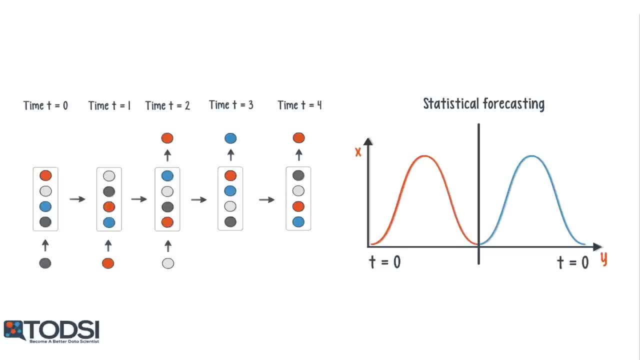 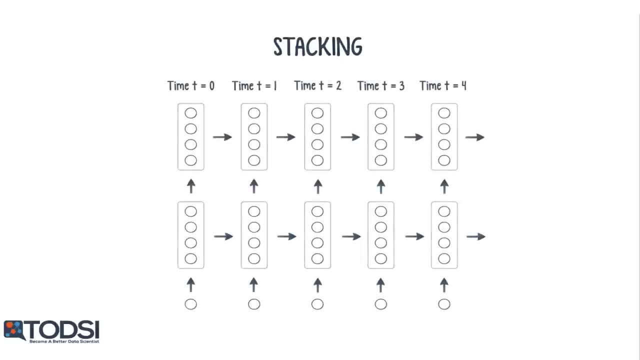 Have you ever used an RNN for one of these applications? If so, please comment and share your experiences. Like we've seen with previous deep learning models, by stacking RNNs on top of each other, you can form a net capable of more complex output than a single RNN working alone. 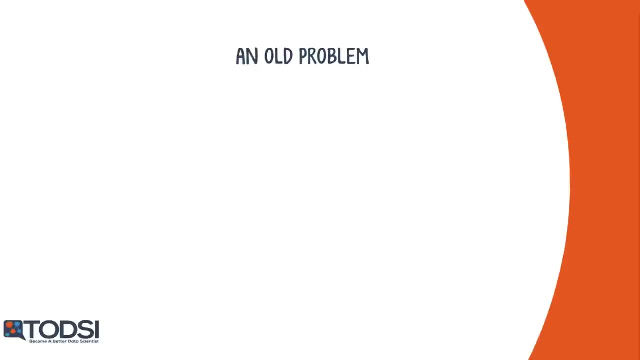 Typically an RNN is an extremely difficult net to train. Since these nets use back-to-back networks, they can be used to track data. Since these nets use back-to-back networks, they can be used to track data. Since these nets use back-to-back networks, they can be used to track data. 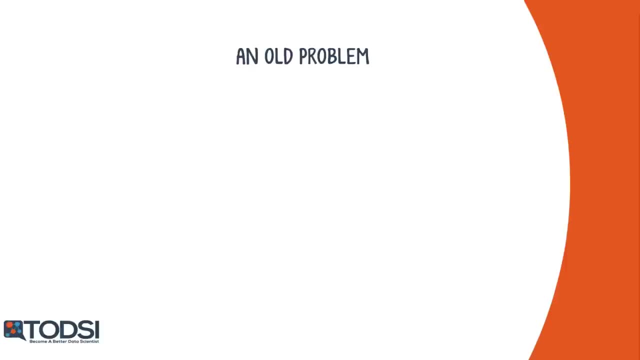 As we've worked on that problem in advanced training and backpropagation, we once again run into the problem of the vanishing gradient. Unfortunately, the vanishing gradient is exponentially worse for an RNN. The reason for this is that each time step is the equivalent of an entire layer in a 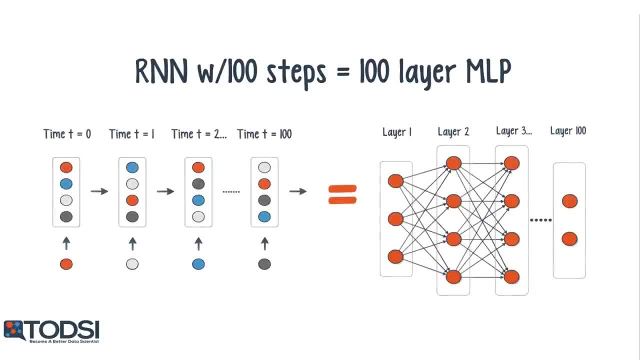 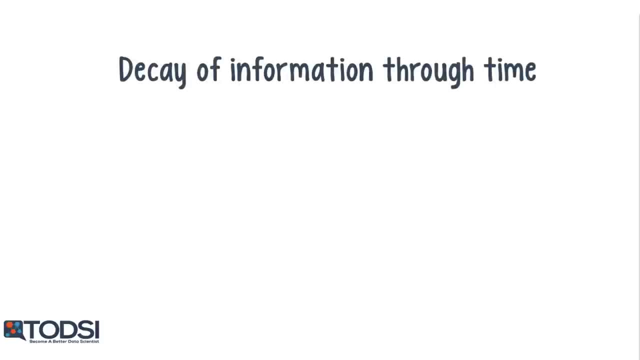 feedforward network. So training an RNN for a hundred time steps is like training a 100-layer feedforward net. This leads to exponentially small gradients and a decay of information through time. There are several ways to address this problem, the most popular of which is gating. 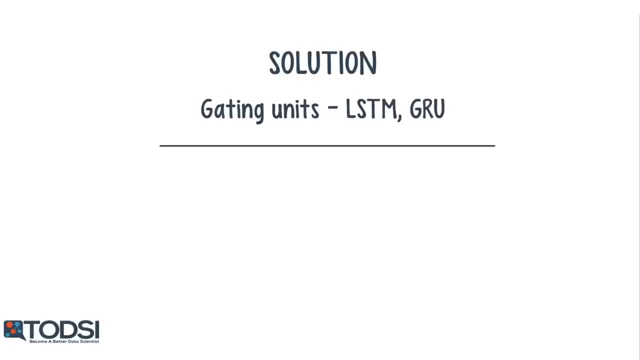 Gating is a technique that helps the net decide when to forget the current input and when to remember it for future timesteps. The most popular gating types today are GRU and LSTM. Besides gating, there are also a few other techniques like gradient clipping, steeper. 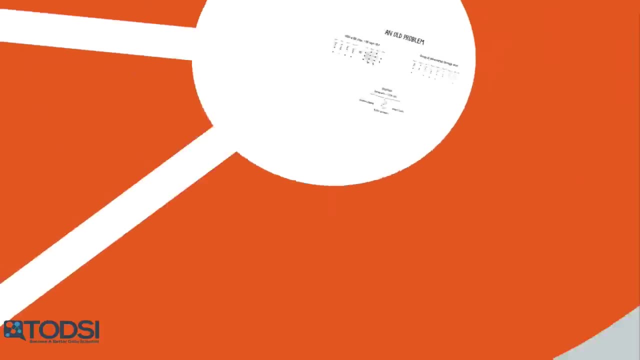 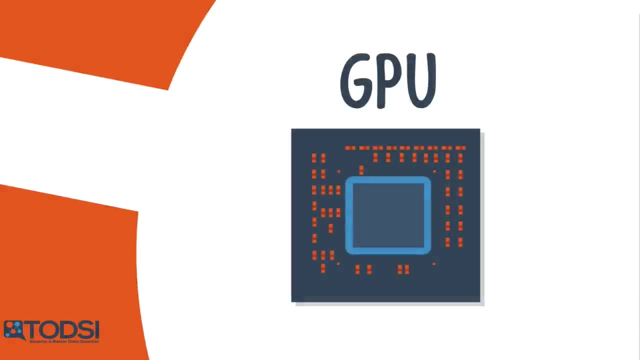 gates and better optimizers When it comes to training a recurrent net GPUs are an obvious choice over an ordinary CPU. This was validated by a research team at Indico, which uses these nets on text processing tasks like sentiment analysis and helpfulness extraction. 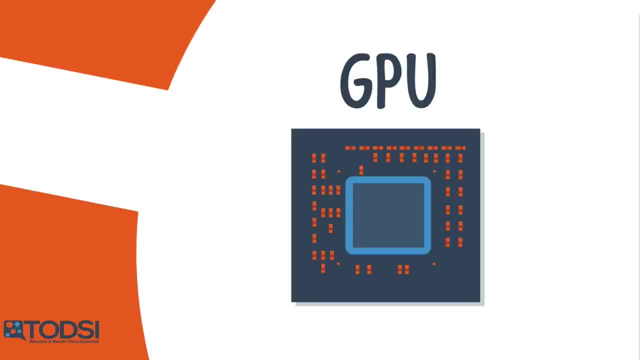 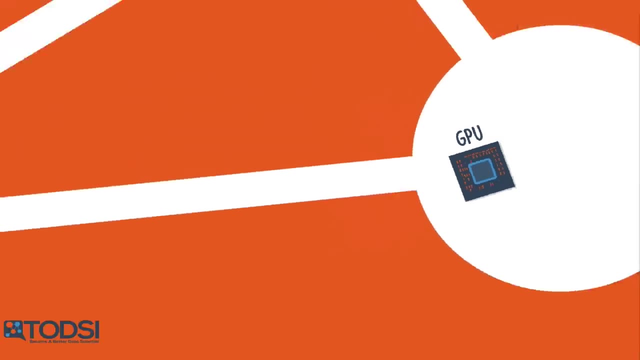 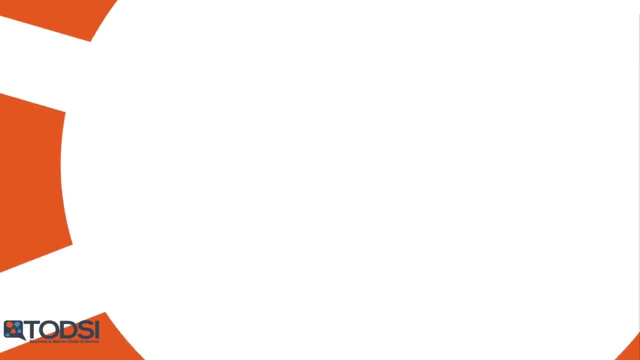 The team found that GPUs were able to train the nets 250 times faster. That's the difference between one day of training and over 8 months. So under what circumstances? So under what circumstances? Under what circumstances would you use a recurrent net over a feedforward net?